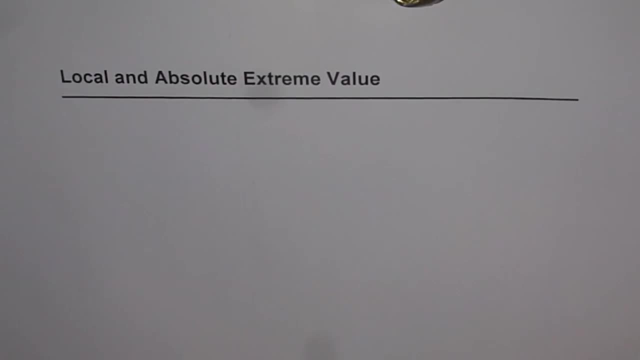 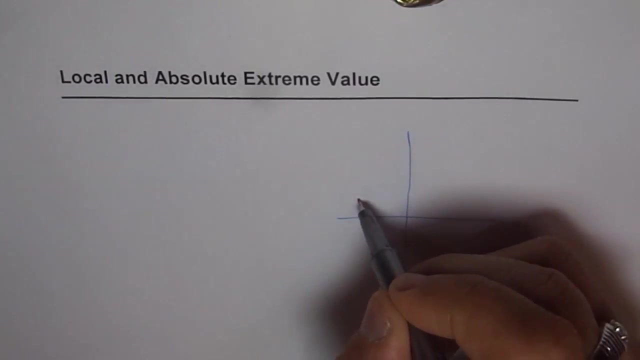 Local and absolute extreme values. So we'll try to understand what do we mean by local and absolute extreme values? as far as the graph of the functions is concerned, Let's sketch one graph and then figure out what are we looking for. Let's say we have a function. 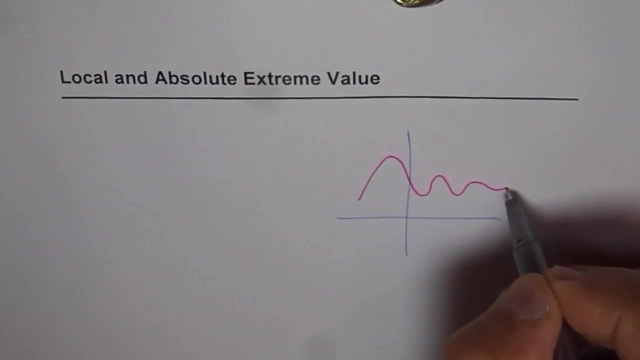 like this and we say we have a lot of peaks in here like this and let's say it stops here and let's say that is our function right Now, as you can see in this particular graph that we have some maximum points here, right, and minimum points. This is maximum, this. 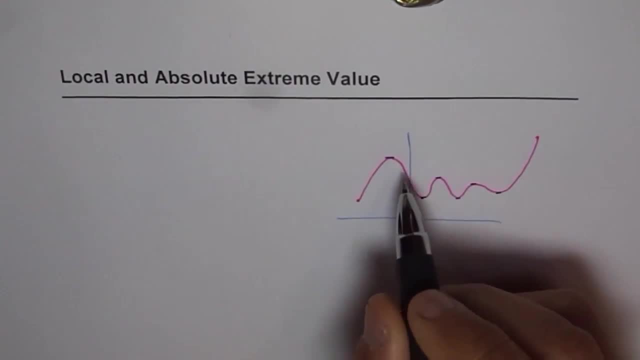 is minimum. this is maximum and this is kind of minimum points, right, This is maximum with respect to its close pi values. do you see that This is minimum with respect to the close pi values in the neighborhood? it is minimum. So, similarly, if you consider, 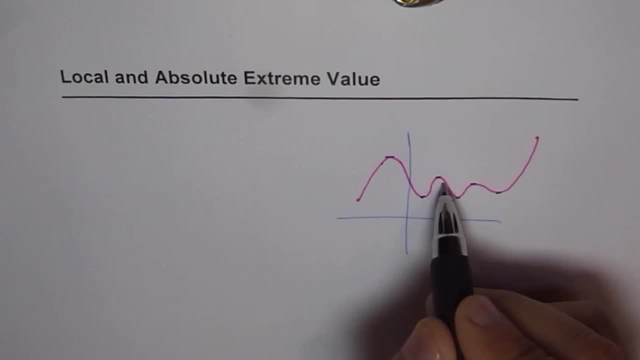 that point. so within our a very close interval, you will find that it is maximum, kind of peaks out and this is kind of goes down in the valley. So that kind of a function, that kind of a graph. when you see for a function, you know those are your maximum and minimum values, but they 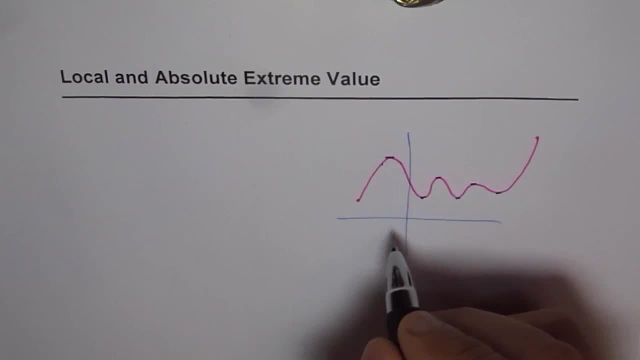 are local, They are like, only for a small, limited portion. So these values which are the lower portions, we call them local minimum values, And these values which you see, like the peaks, they are local maximum values. Right, And also you find that, as far as the 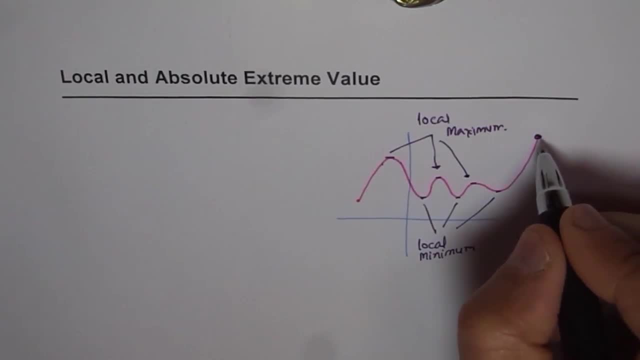 function is concerned, it does have a maximum. This, this is like there is nothing more than that during the whole graph which you see here. So we'll call this a minimum, We'll call this as absolute maximum. Similarly, this one seems to be the lowest point. So 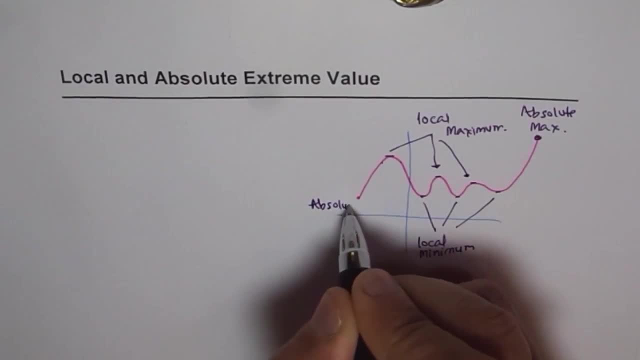 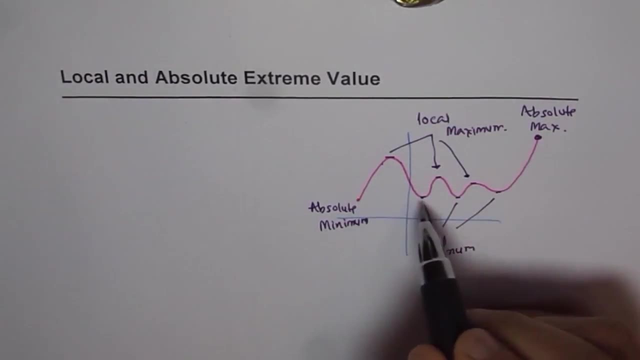 this is our absolute minimum, Right. It is not necessary to have absolute maximum minimum at the ends, Right, It could be at the center also. You've seen graph of a parabola, for example. Right. So we have absolute minimum and local minimum- same also. 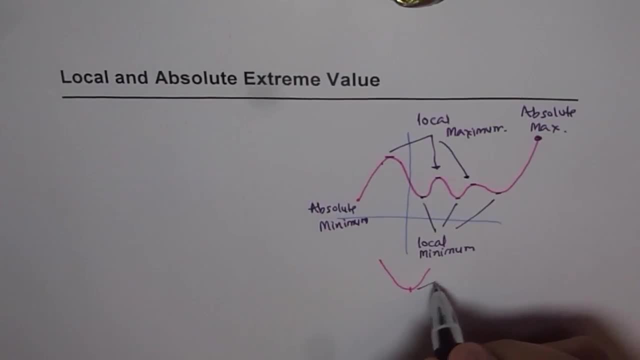 So there is a possibility of both being same. also, We have same absolute and local minimum in this case, right, So so that is possible, correct, And what we notice most of the time is that these local maximum minimums occur when they. 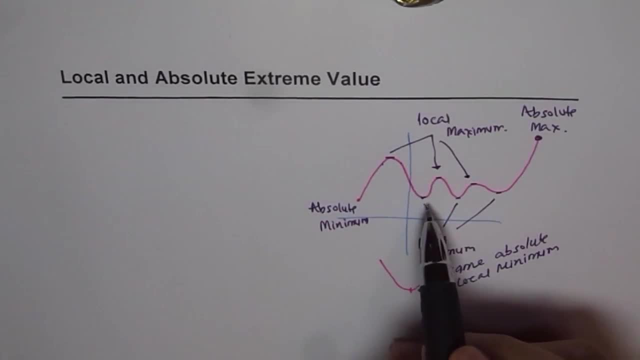 are the turning points. So whenever the graph turns, so what we're seeing is whenever changes from increasing to decreasing, I mean we have a whole bunch of values on the graph decreasing, then we have maximum, and when it changes from decreasing to increasing. 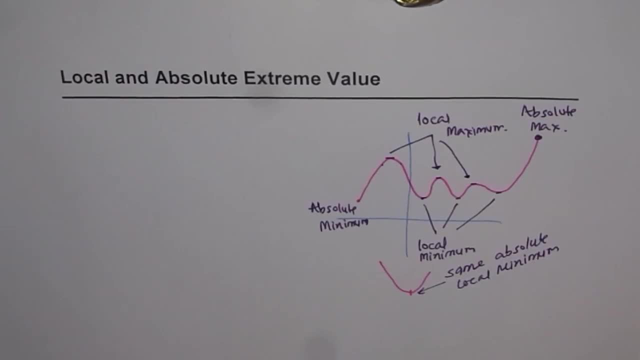 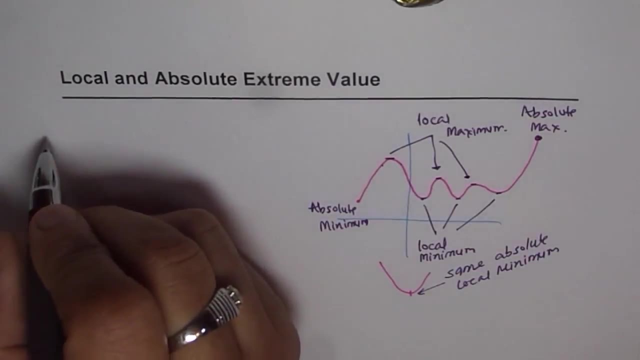 then we have minimum right. That is one way of looking at it, right. As far as the functions are concerned, when we talk about increasing and decreasing, so what in function, when we find derivative, if the derivative is greater than zero, then 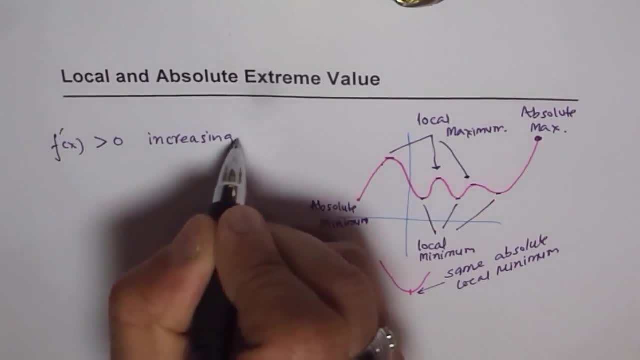 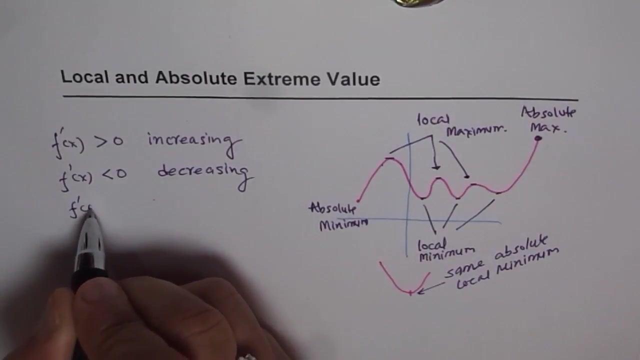 we say function is increasing right, And if the derivative is less than zero, then we say that the function is decreasing. So basically, if we try to find a point where derivative is equal to zero, then we know it's a critical point. 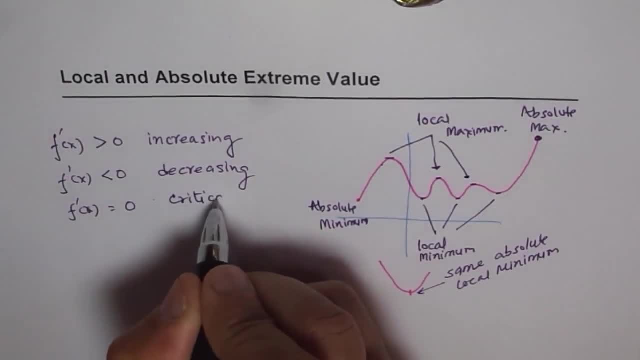 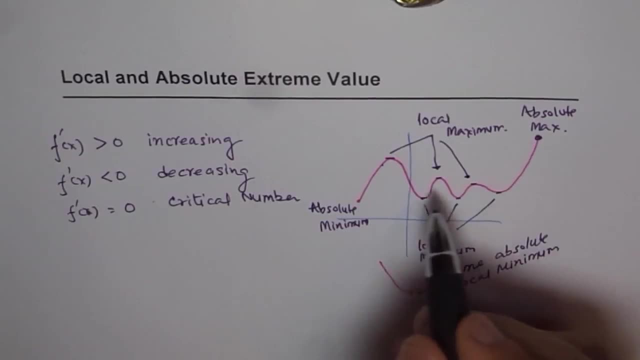 We call that as a critical number, right, or a critical point. So in this case, if you find derivative of the function, you'll find that these are our critical points, right. So, and if you observe what happens to the derivative before and after, 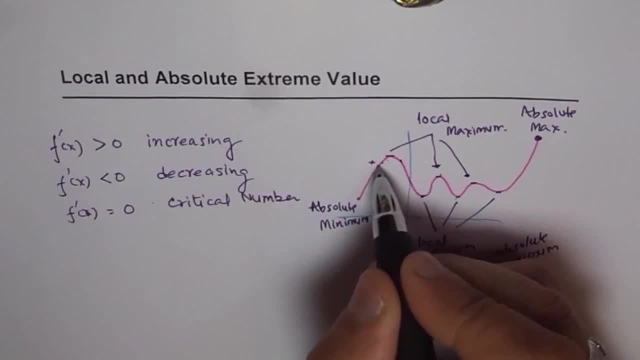 So in this case, before it is plus right, So it is derivative I'm talking about. so it is increasing and then it is decreasing. Since it changes from increasing to decreasing, we have a local maximum and in this case, 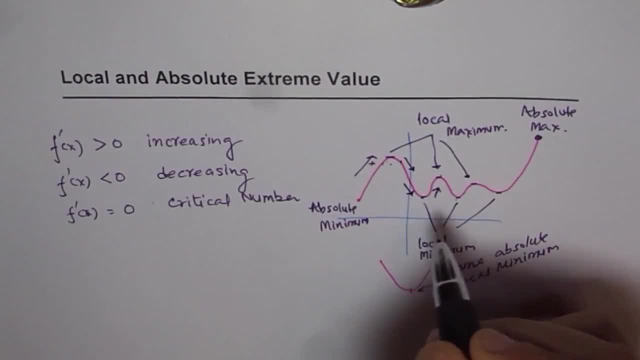 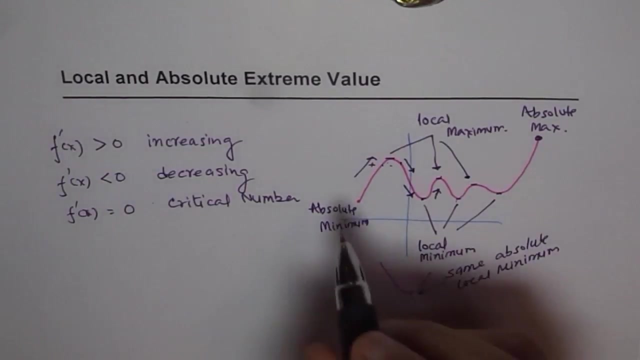 it changes from decreasing to increasing, So we have a local minimum. So that is another way of algebraically finding, with the help of derivatives, the points on the function graph where it could be increasing or decreasing right Now. the other things are the end points of the function, right. 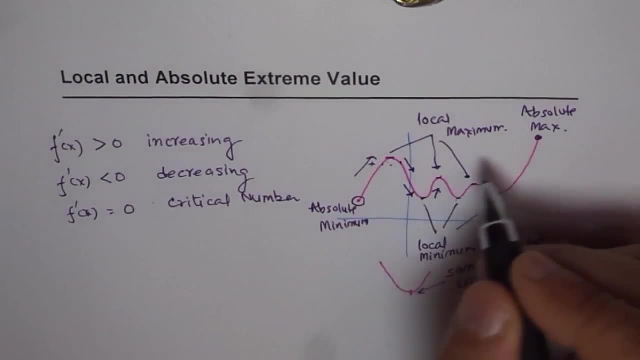 So at the end points we could always have absolute maximum minimum right. There is a possibility that this function could have been the lowest most point, So a local maximum minimum, as you can see here, could be also absolute maximum minimum right. 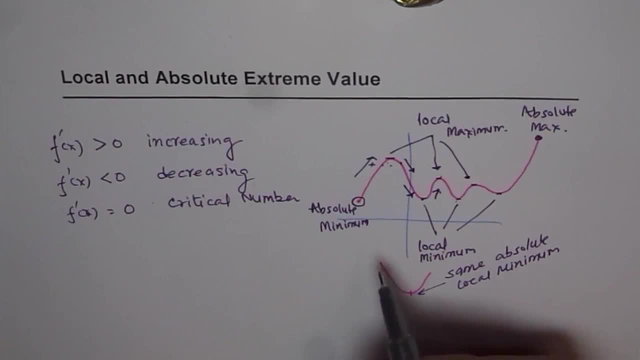 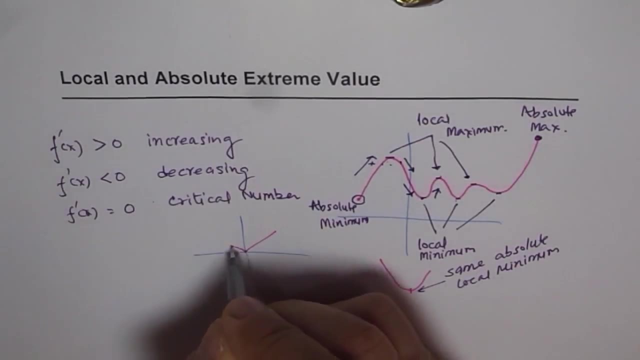 There's one more critical case which I would like to highlight here. At times you can have functions which are, as you have seen, absolute function right. So in this kind of a function, if I find the derivative, then I know f dash 0 does not. 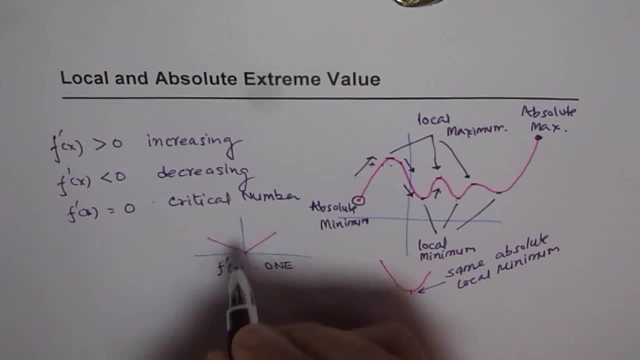 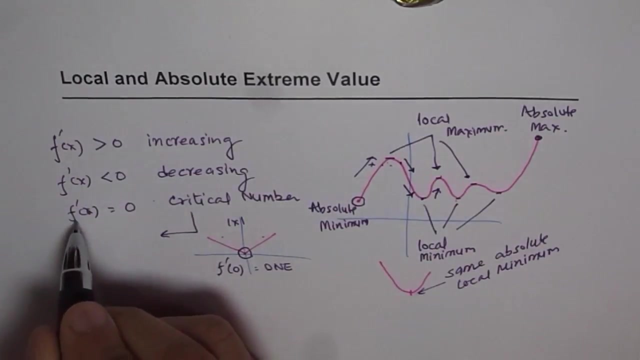 exist, right, The derivative is 1 here and negative 1 here for absolute x. but it does not exist at this point, correct? So that is all. See you next time also a critical number. so for critical number we have two criterias. one is f dash x is equal to zero. 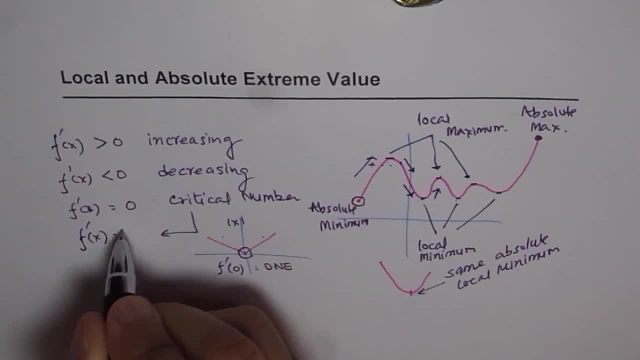 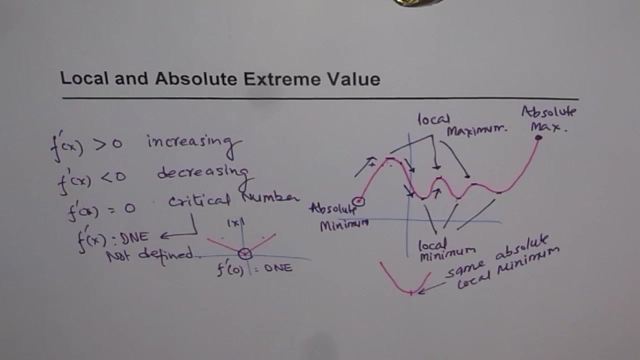 and the other one is f, dash x does not exist, right is not defined, is not defined. so that is in the criteria. now getting back and combining all these things is that when we are looking after the points which are, which could be absolute or local, extreme points, that means maximum or minimum- then the way to go about is to find the critical numbers. 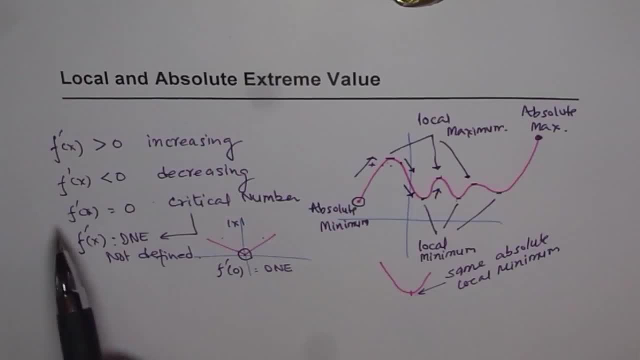 a critical number is a point where the derivative of the function is either zero or it does not exist. then, once you get the critical points, you can actually find whether it is increased, change from increasing to decreasing or decreasing to increasing in the neighborhood of that point. right, if it changes, then you have a local maximum or a minimum. right now, another criteria which you 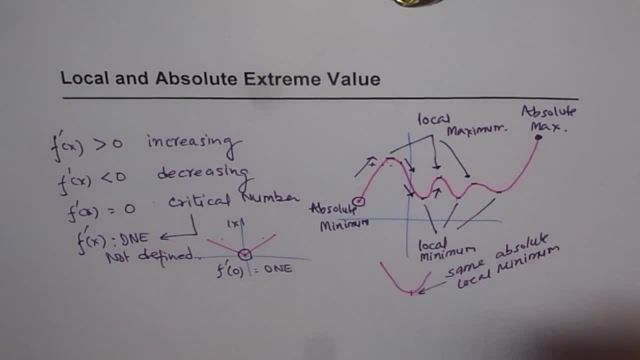 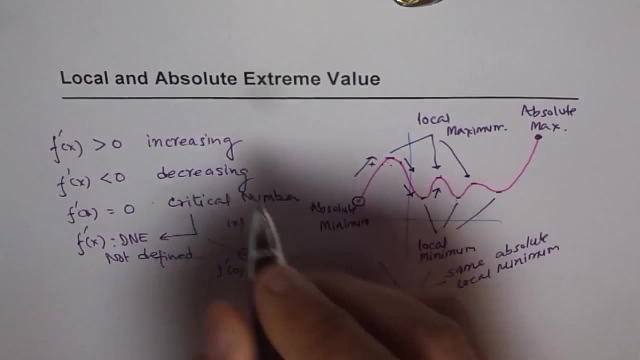 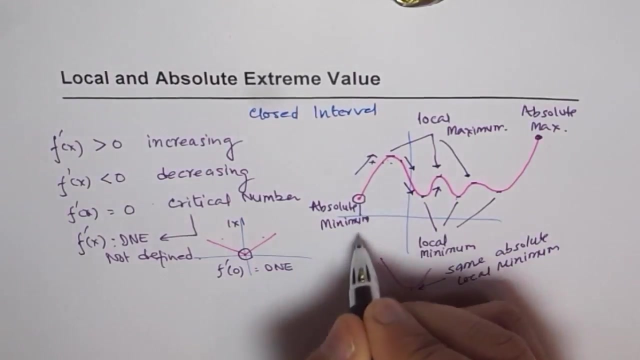 find is the boundary of the condition right. see, one more analysis is to be done with respect to the boundary right. so we call this as a closed interval. let's say: this point is that x equals to a and this point is that x equals to b. then we will say: